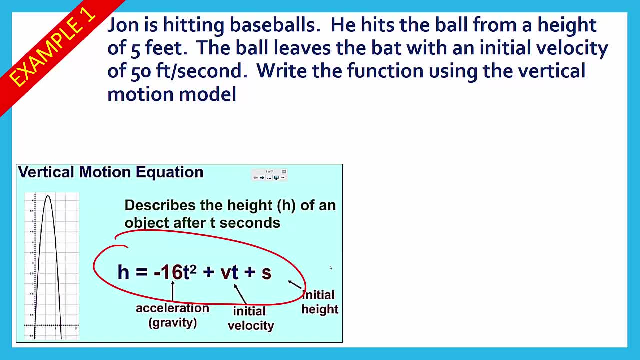 or gravity, depending on the problem. So, generally speaking, if there's nothing there, we're going to have it as a negative 16, unless the problem specifies otherwise. v is always going to be your initial velocity, s is your initial height And then h is your height. 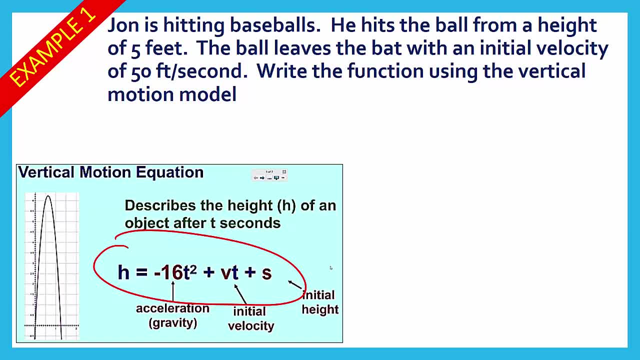 at any given time. So if I say like after three seconds, and I plug in three for t and get an answer, that would be the height at three seconds, But all we have to do is write a function. So all we're looking for is when gravity or acceleration is not mentioned and initial velocity is. 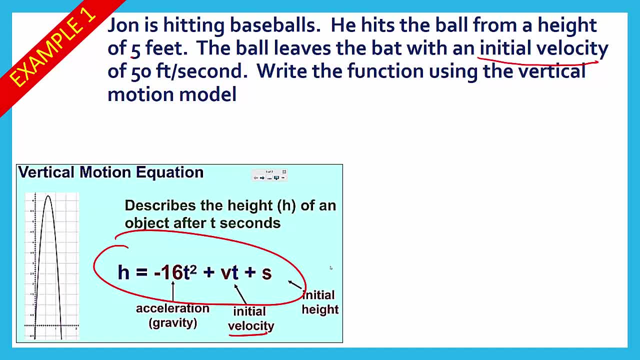 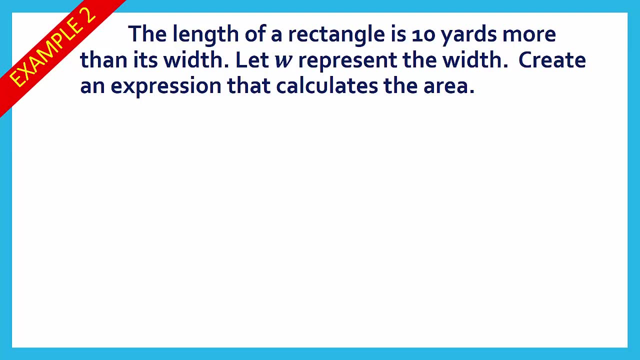 which notice that's going to go in for v, And then our initial height of five feet mentioned. Okay, so we just plug those in to get h equals negative 16t squared plus 50t plus 5.. Next problem: The length of a rectangle is 10 yards more than its width. Let w represent the. 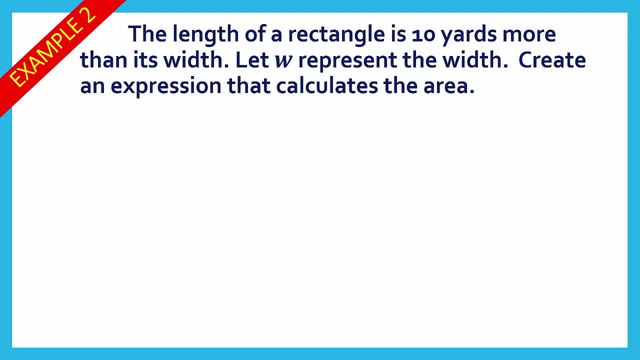 width, Create an expression that calculates the area. So, before you do this, you need to remember the formula for area, which is width times length, base times height. however you want to look at it, In this problem we're talking about width and length, though we're going to use those, So our 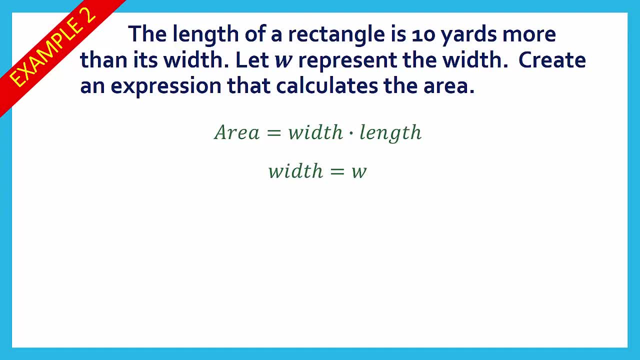 width, we're told is w. Okay, our length. we don't have an exact variable for We just know that it's 10 more than its width, So we can write it as length equals our width plus 10, because it's 10. 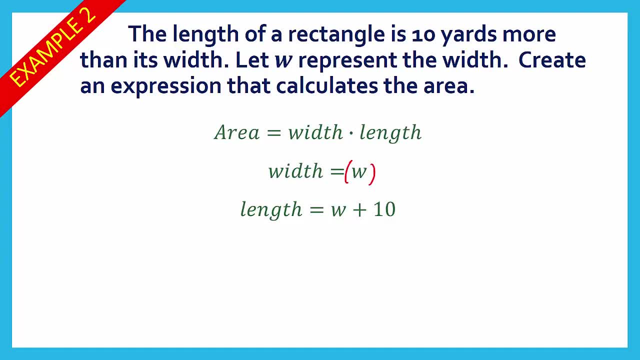 yards more, So we can plug these two expressions. We've got w and w plus 10, because, notice, it's width times length, So I can tie. I can have my answer as a for area equals, w which is the width times the length, which is w plus 10,. 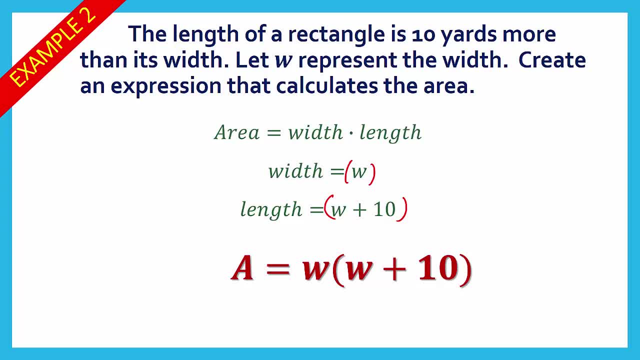 and make sure to put that in parentheses. You don't need to do anything other than that either. I mean, if you really wanted to, you could expand it and get w squared plus 10w, but we're not going to ask you to do that. Third example: A ball is thrown straight up from 7. 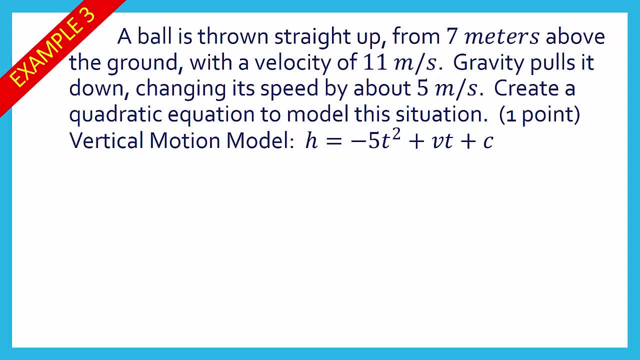 meters above the ground with a velocity of 11 meters per second. Gravity pulls it down, changing its speed by about 5. meters per second. Create a quadratic equation to model this situation. Okay, vertical motion model again. So notice this change to a negative 16.. So we kind of gave you that, but the thing. 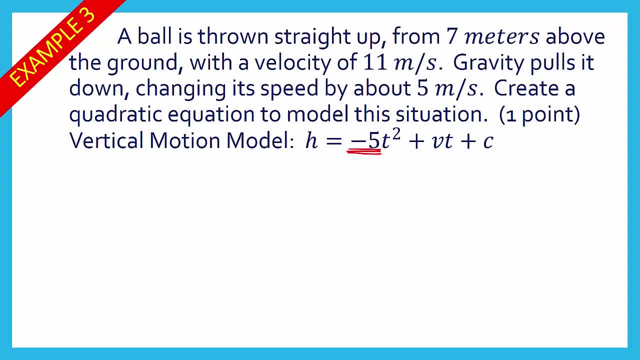 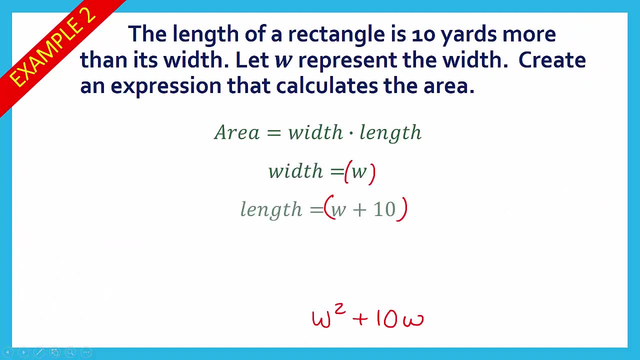 to remember is this minus 5.. Okay, this is gravity, pulling it down- hence the negative- by about 5 meters per second. So that's where that 5 comes in. So that's already been put in for you. but the thing to remember is, if we go back to this, this is acceleration or gravity. 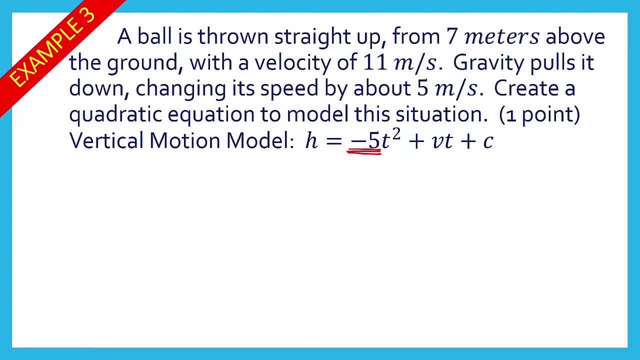 So, since you see that word gravity mentioned, hopefully you can make that connection which only leaves the initial velocity and its starting height. Okay, you might not always have a starting height, in which case this would be left off, Like if you have a if, whatever it is. 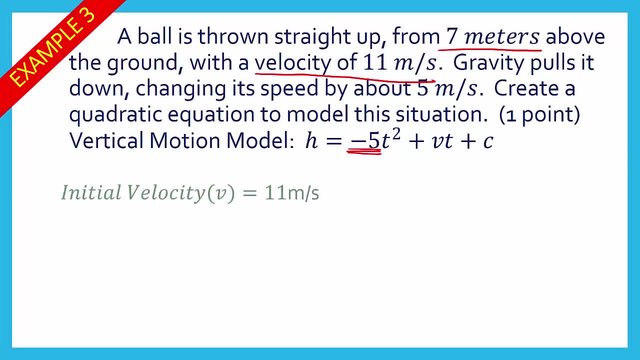 is starting from the ground, then you won't have a constant in there. But as it is, our initial velocity is 11 meters per second. starting height, which is c, is 7.. So we just plug those in and we are good to go Next. All right, 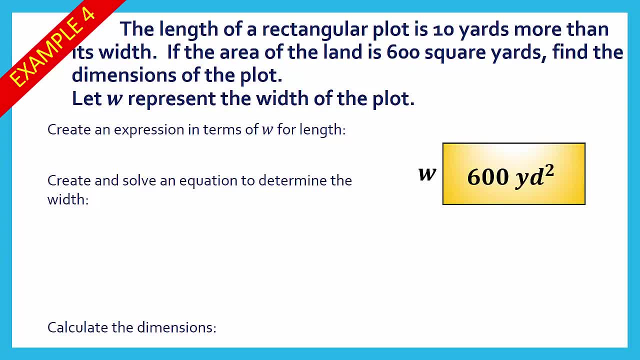 Length of a rectangular plot is 10 yards more than its width. If the area of the land is 600 square yards, find the dimensions. W represents the width. Okay, so there's w, that's our width. We want to create an expression in terms of w for length. So the thing to remember here. so if this is our, 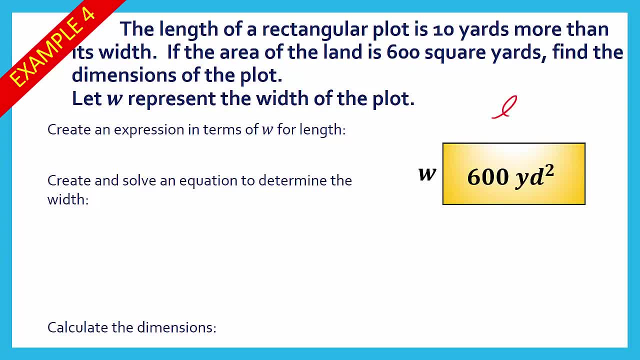 length, our width. this is our length, right here, All right, and we've got to go and look. It says our length of a rectangular plot is 10 yards more than its width, So we can write it as w plus 10.. For those of you who want a visual, this is what it looks like: Create and solve an. 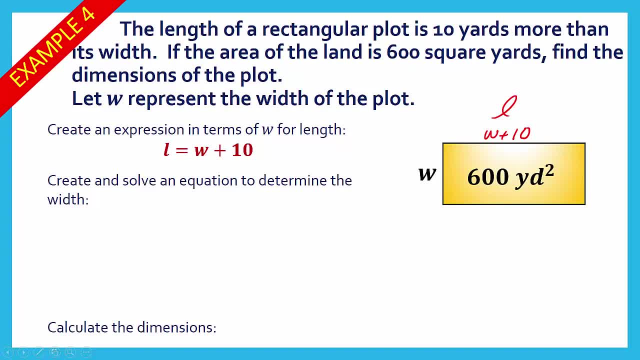 equation to determine the width. Well, if we're going to determine the width, then we're basically solving for w, So we're going to set it up w times: w plus 10.. Now notice, I have 600 here, not another, not a variable. That's because this is the formula for area. 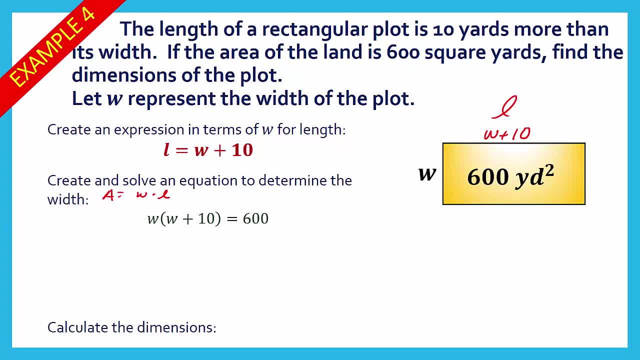 is width times length, But in this case I'm just switching the side, So it's width times length. Length equals area. Well, I know that the area of the land is 600 square yards, So that's where I got this. My length is w plus 10, and then width is a w, So now I'm just going to go ahead. 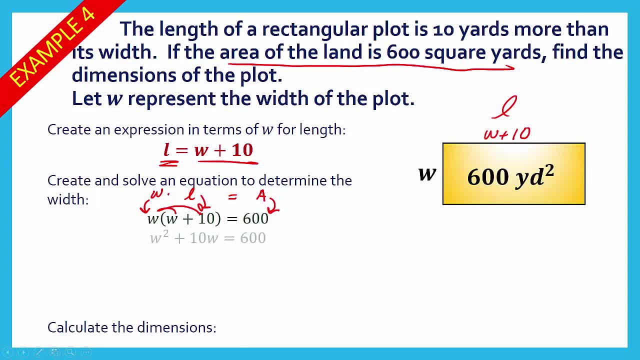 and distribute this: W times w is w squared, W times 10 is 10w and 600.. And to make this a proper quadratic, we're going to subtract 600 from both sides to give us w squared plus 10w. 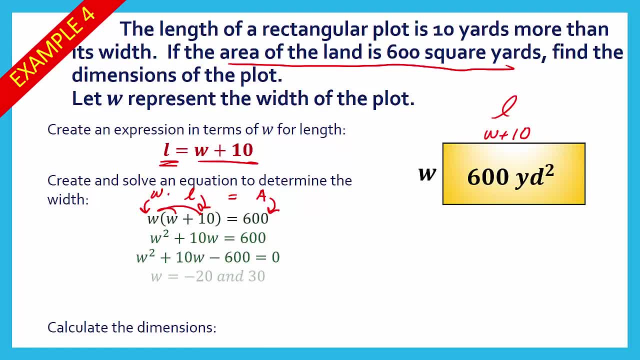 minus 600.. Now we have it set equal to zero And now we can subtract 600 from both sides. So we're going to solve whichever way we want. Okay, you can solve by factoring, You can solve by the quadratic formula, You can solve by using a graphing utility, So it would just say graphing. 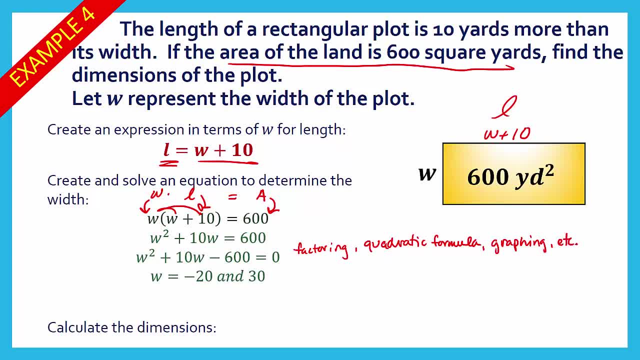 Okay, you get the idea. There's lots of different ways that we can solve this. You choose whichever one works for you. You're not told to solve it any particular way, But this we solve and we get two w's. or if you're using a calculator, you get two w's, So we get two w's. 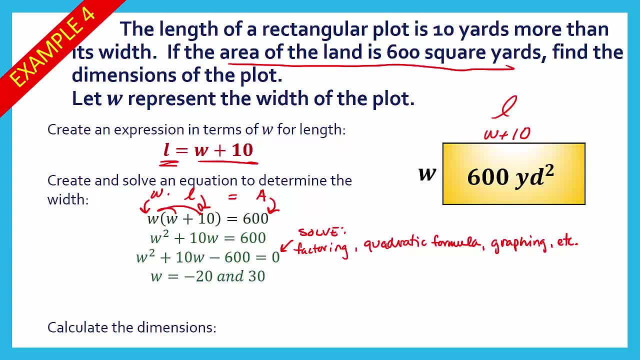 You might have to put it as x's of negative 20 and 30.. Now remember, our width is just w. We can't have a width that's a negative number, So we don't include that. We don't include negative numbers when we're talking about real world problems. So all we're left with is w equals 30.. Now we need 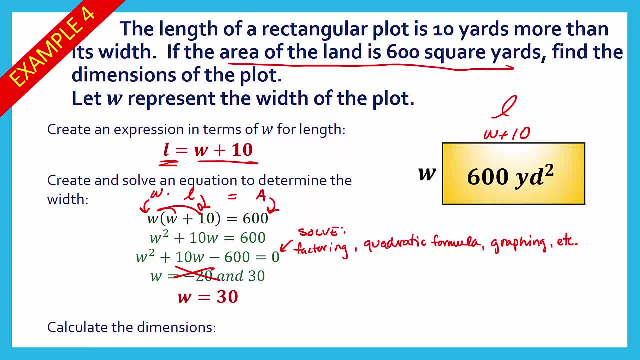 to calculate the dimensions. We know that the width is 30, but we don't officially know the length. But it's easy enough to find out because we do know the length is 10 more than the width, giving us a width of 30 yards and a length of 40.. 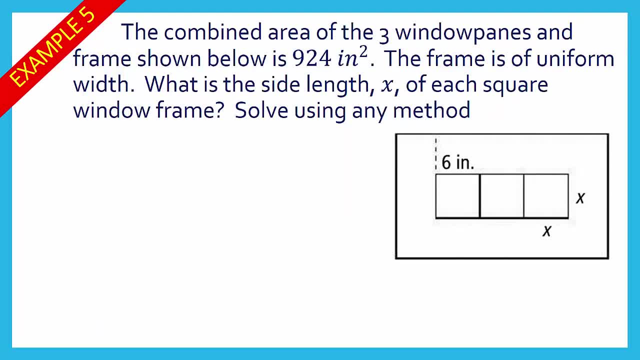 All right. last problem of the last target of this unit. Okay, the combined area of the three window panes and frames shown below is 924 inches squared Nine 924.. Sorry, The frame is of uniform width, meaning it has the same width This space around. 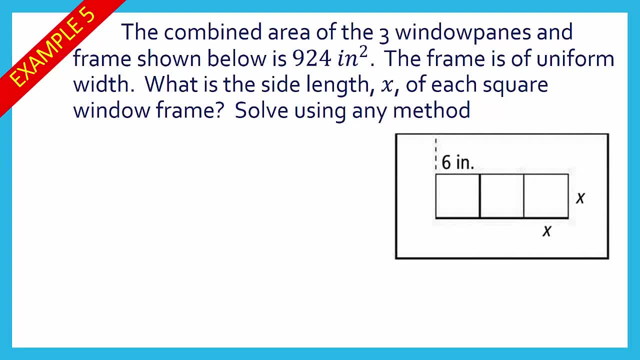 the three window panes is the same all the way around. What is the side length? X? So we want to know the side length. Just this right here. Okay, Because each of these sides is the same length, because each window frame is a square, So each side length is the same. Solve using any. 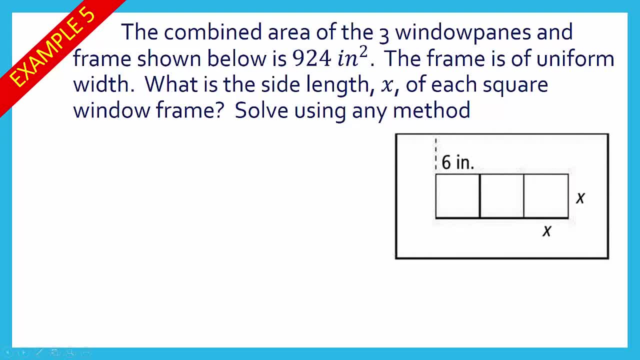 method. All right. so the thing that I want to kind of like set up here for you is to remember, and you might want to do this: that's six inches, That's six inches, This is six inches. Now you might be wondering: why am I doing this? 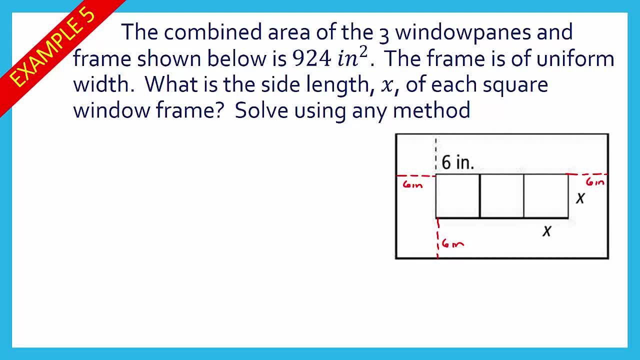 Not everywhere. Well, if you notice, I've got a line here and a line here, So what we need to do is set it up so we have area. again is width times length. The width is 3x plus 12.. I'm telling you that right now. Take a minute, see if you can figure it out before you. 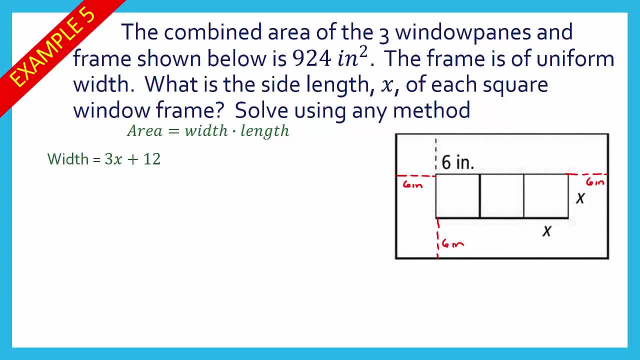 continue. But again, all of these square panes are uniform, which means this has a length of x, this has a length of x. So how many x's do we have? The three of these together are 3x From here to here. Okay, so we have 3x here, and then 6 and 6 is 12.. Oh, look at that. So now that. 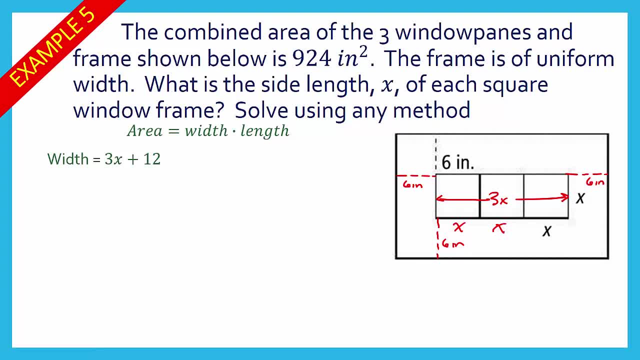 you know that. what do you think the length is? Well, hopefully, and if I get it backwards it really doesn't matter. You can again see 6,, 6,, but this time we have a distance here of just x. 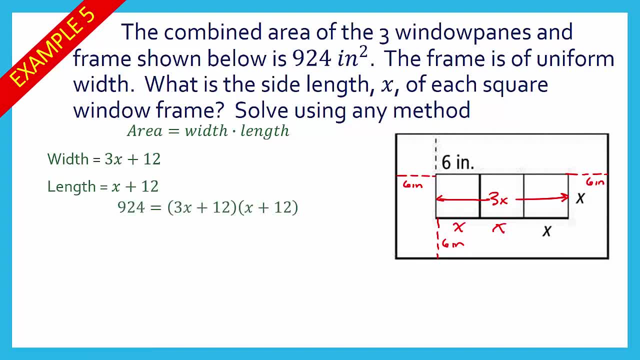 so we have x plus 12.. And then we multiply the two together and we set it equal to 924, because we know that the area is 924.. So we get 924.. So we have 924 plus 12.. We get 924 plus 12 plus 12.もう. 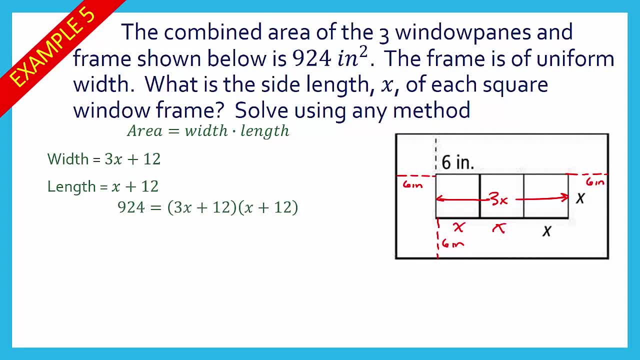 nine, twenty-four, because we know that the area is 924, and we know that the area is 924.. So we get 924, because that's including the frames. all right, so we multiply those together. use foil to get 3x squared plus 48x plus 144, then subtract the 924 from both sides so that you can set this.